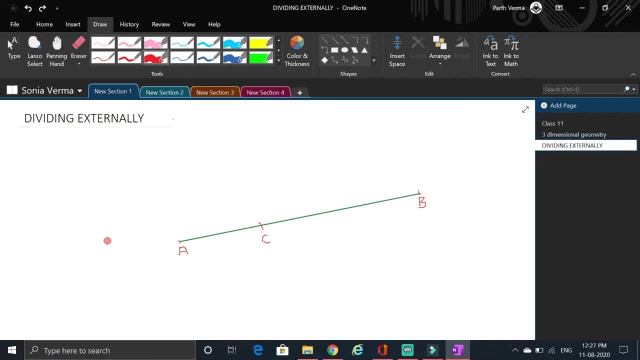 can it divide a line segment by being outside? but it is so. And what is the significance of ratio in such a case? Just understand that. Let us take the example of this. Suppose you have the line segment C, B- Okay, this one only. And suppose A is dividing this line segment in the ratio to ratio 5.. 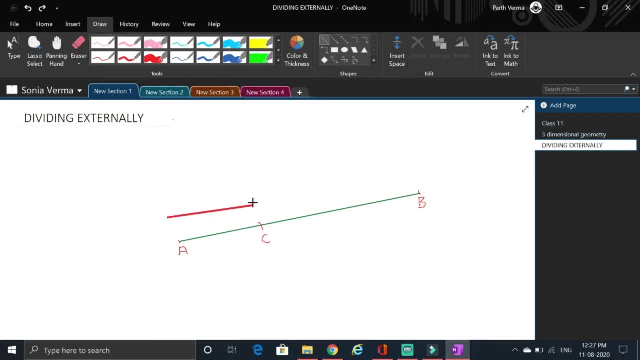 That this is 2 and this is 5.. So A is dividing C, B in the ratio to ratio 5.. Okay, Sorry, So as C comes first, so AC is 2 and AB is 5.. And A divides BC in the ratio 5 ratio 2.. 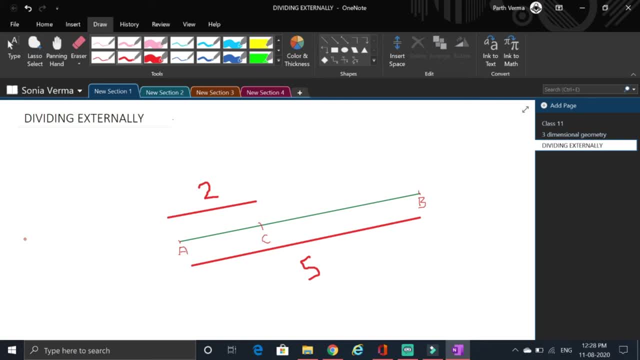 This is the actual meaning of external division. So whenever you have been given such a question that a point divides a line segment externally, So there are two things to be note down there: that the point lies outside the line segment and is collinear with the line segment. 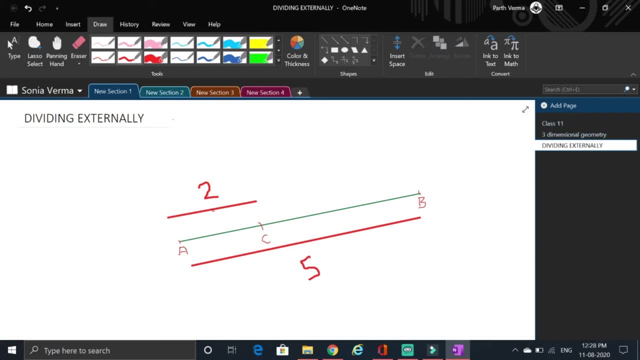 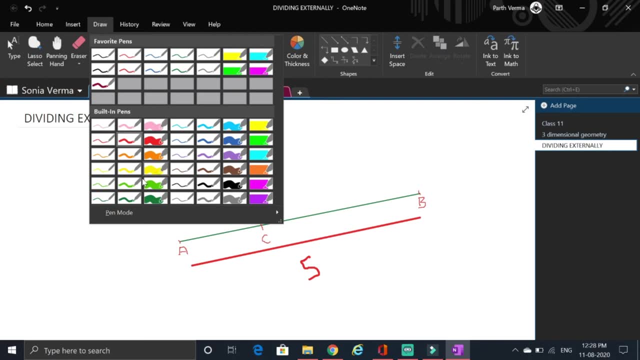 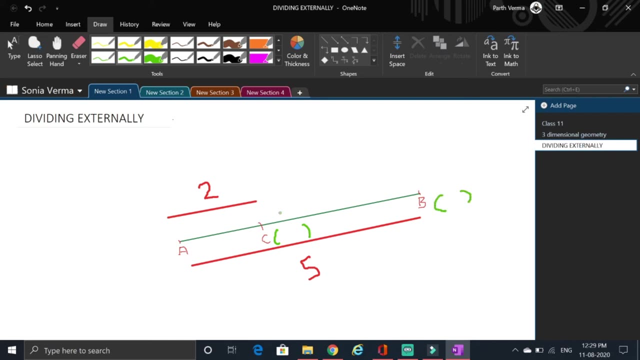 Okay, And you can interpret the ratio in this way, as I have done here. Okay, Now, if you have been given the coordinates of the points- these means the endpoints of the line segments- then you should be able to find out its coordinate by using this ratio. 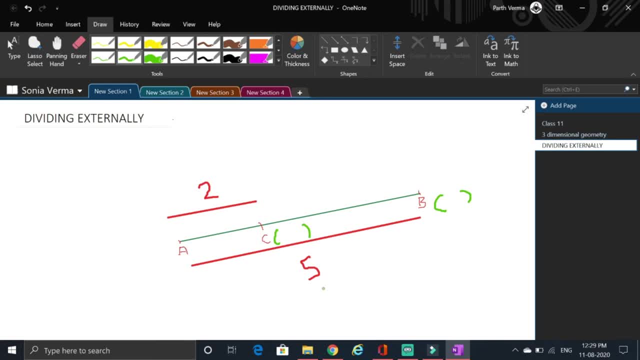 of 2, ratio 5.. Either you have to create a new formula for this, Okay, Either you have to create a new formula for this, as we generated for the section formula, as we generated the section formula for the internal division, or you may use the same. 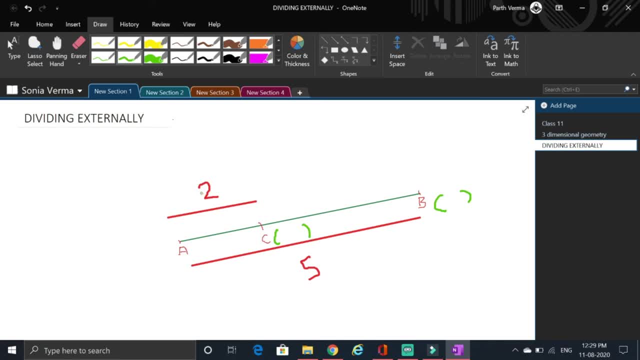 formula, How come You may, as this is 2 ratio 5, then you can say: this is 2 and this is 5.. Sorry, 3.. So now this actually became 2 ratio 3 and you can say: C is internally dividing AB and